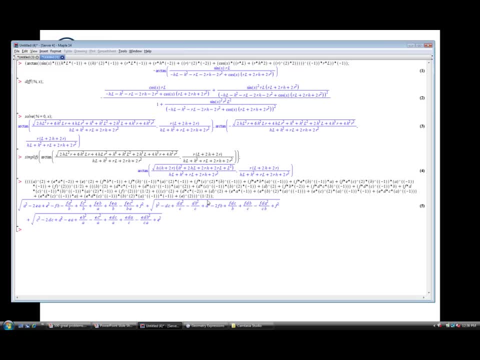 It's D, E and F, the location of the three different points on that inscribed triangle. And so, to find the minimum we'd like, we want to find A, We want to find values of all three, of those which give an absolute minimum. 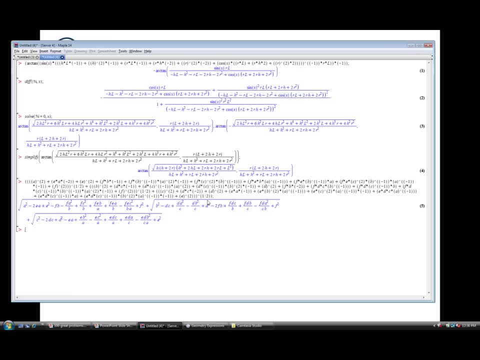 So we'd like to. what we need to do is differentiate with respect to all three of them And find a location where all three of the derivatives are zero. So let me do that. We'll call the three derivatives Dx, not Dx, Dd. 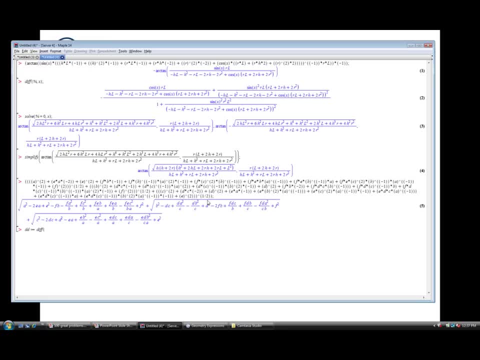 There's the derivative. There's the derivative of. actually, let me just back up here. First of all, let's give a name to that perimeter. We'll call it P. P is the above. Now, first of all, I'm going to take: let's just call it D P. 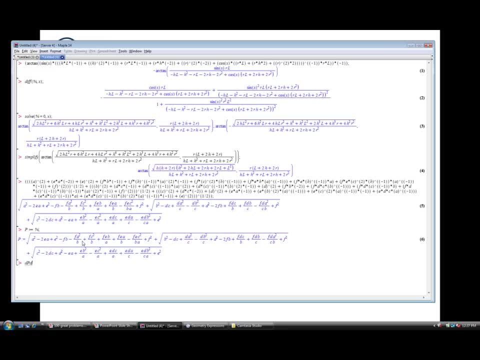 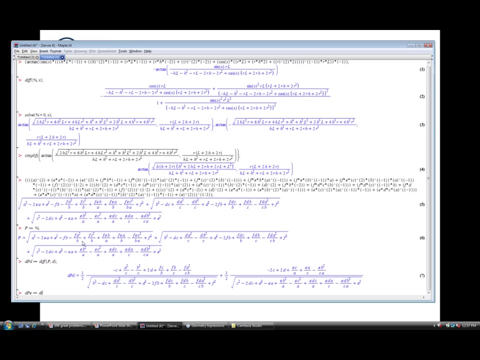 We'll call it D P D. There's the derivative of P with respect to D, And that's going to look like that: D P E, The derivative of P with respect to E, Going to look like that: 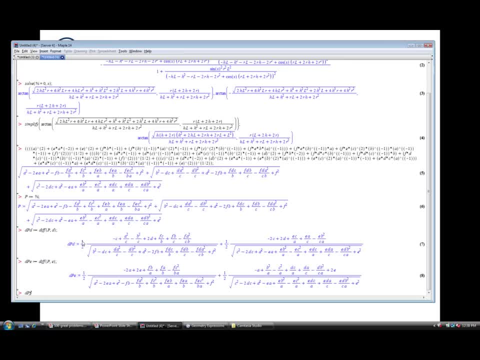 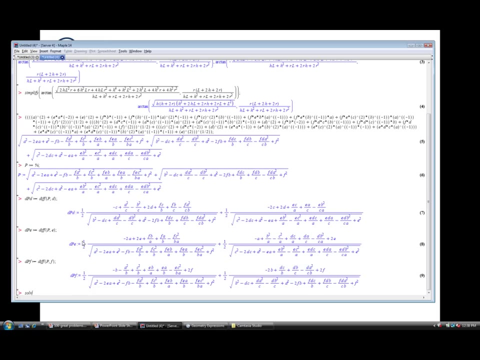 And D P F, The derivative of P with respect to E, Going to look like that. So what we'd like to do is solve three things: D P D. D P D equals zero. D P E equals zero. 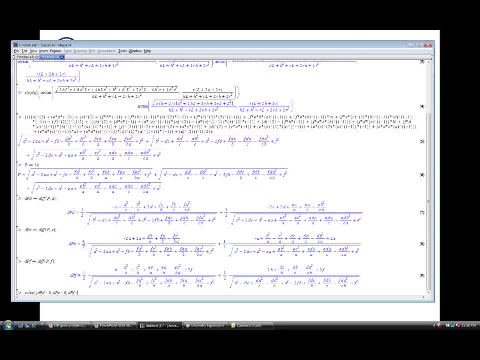 And D, P, F equals zero. So solve all of those three things equal to zero For three variables: D, E and F. Now Maple is going to take a little bit of time for this. Last time I measured it, not too much time. 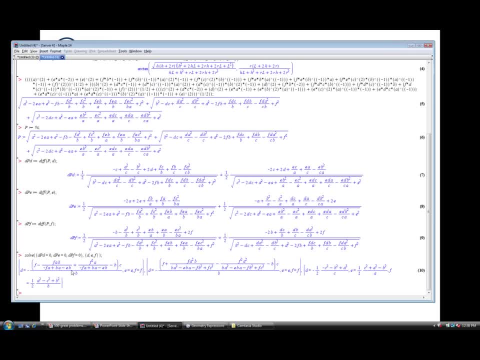 We can see there are. there's one solution here, One solution here, One solution here. We've got three different solutions. Now these solutions- the first two solutions- have E equals E, F equals F. So there are solutions that are true for any value of E and F. 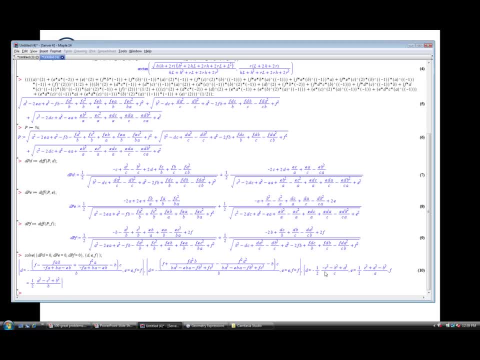 I'll look at that in a second, But let's look at the third solution. It looks pretty interesting. It's got a specific value for D, a specific value for E and a specific value for F, So let me just grab that. 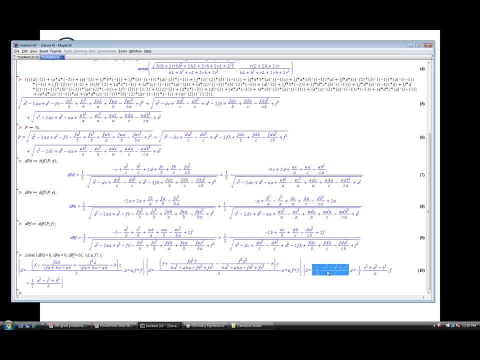 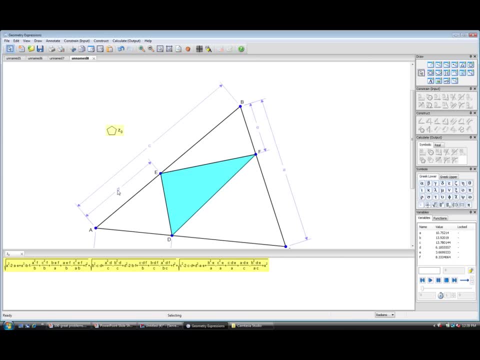 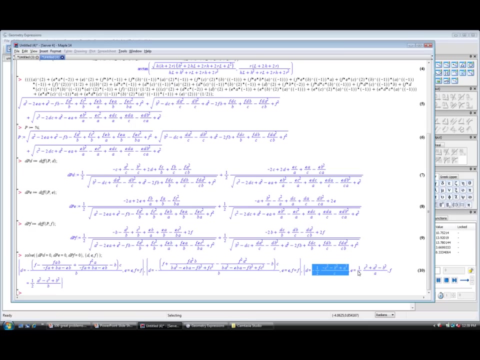 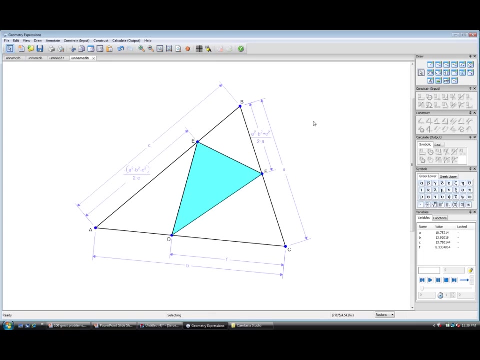 So grab it piecemeal. First the D part. So we'll replace D by that. I don't really want it to keep computing the perimeter every time I do that. So that's that's my D. Grab the E part. 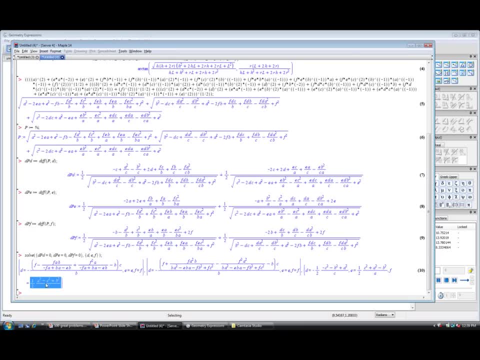 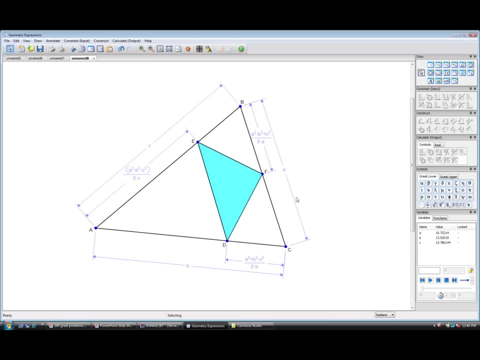 And let's grab the F part here, And so there is my minimal location. Let me just- well, actually I haven't proved it's minimal, I've proved it's either a maximum or a minimum, And that's another thing to do. 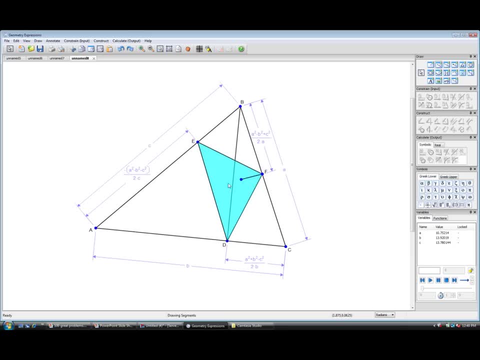 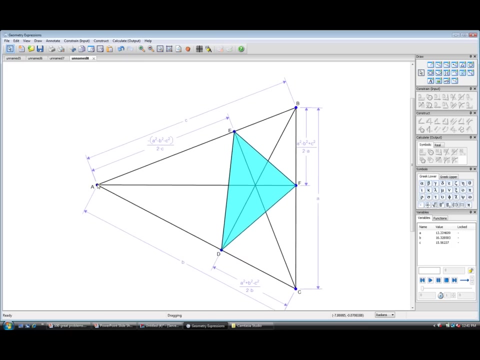 But let me Just draw the lines which are connecting the vertices of my inscribed triangle And as I change the original triangle, do you notice anything about those three lines? There is something to notice if we ask for the angle between the line and the opposite side of the triangle.